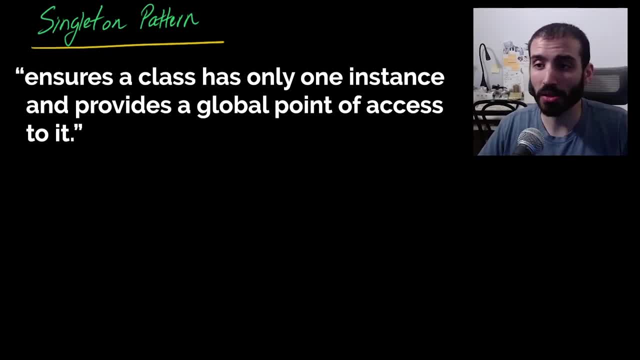 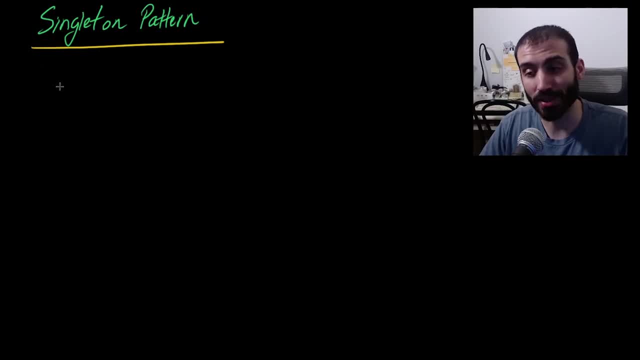 you're just getting into software. So that's the definition of the singleton pattern. Let's talk about why it's useful. So, in terms of why the singleton pattern is useful, there's two main buckets of reasons why it's useful. The first one is it allows for what's called lazy loading. lazy loading And what that essentially 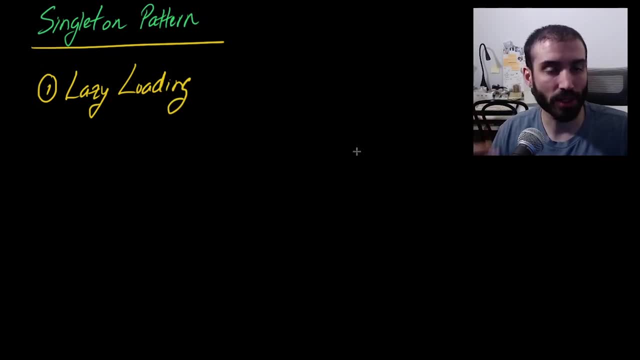 means is that lazy loading allows you to do is basically initialize your object creation only when you need it. If you were doing it through, like using a global variable or something that's going to happen at the initialization step of the JVM. So with lazy loading you don't have 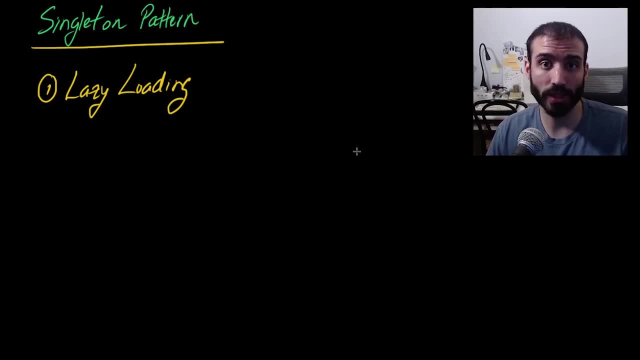 to initialize and create an object unless you're actually going to be using it. So that's one of the benefits of using the singleton pattern. The second main benefit is when you only really need one instance. So you only really need one, Need one. And what I mean by that is like, how about something like a database connection? 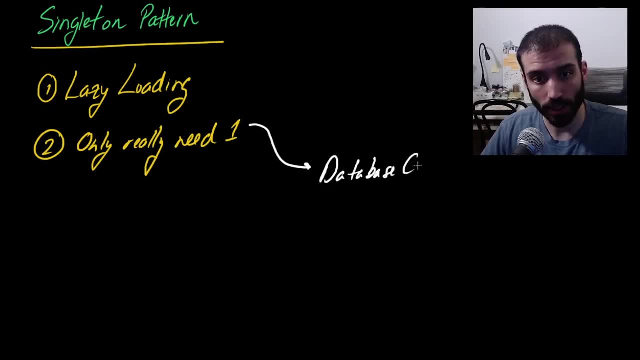 Database connection. Maybe in certain applications you want to only have one database connection, or you kind of want to restrict the number and restrict the number of database connections through a class, So you only want to have one instance Of that. So that's one kind of potential application of when you only really need one of. 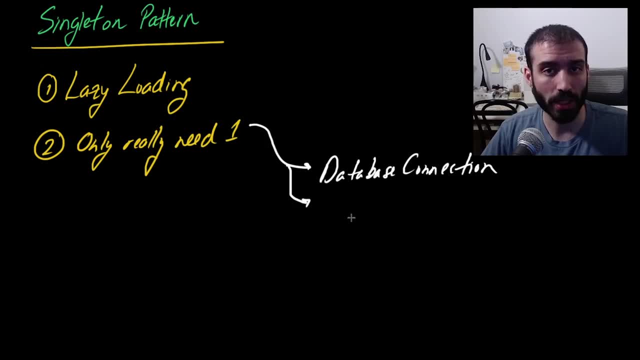 an object. The second one, a little bit more abstract but kind of an interesting thought exercise, is like what if you're building a kind of a rocket ship guidance system, rocket ship guidance system, And so you know it only makes sense to have one instance of the 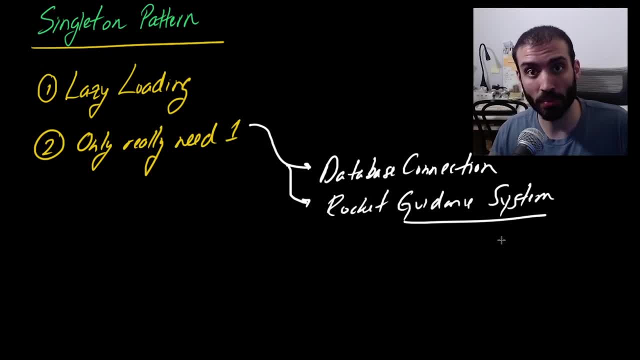 guidance system initialized at any time, because this guidance system could be performing actions on the physical hardware that exists in this rocket ship. So you don't want to ever accidentally initialize two because maybe they'll be sending conflicting instructions to the actual hardware. So those are some of the applications of using it in the 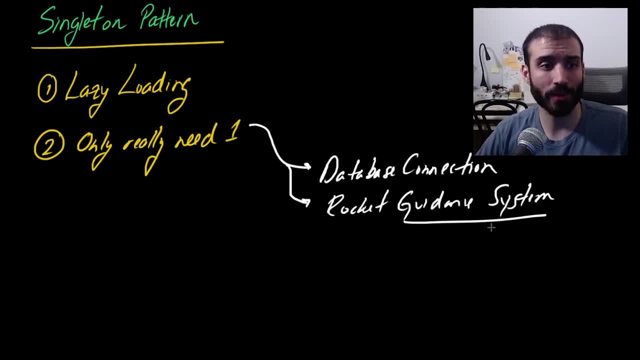 real world. Truth be told, the singleton pattern is probably the most simple design pattern. It's only like maybe 10 lines of code, but it's applications are everywhere and you're always going to be seeing it. So we talked about why it's useful. Now let's get into some of the mechanics. 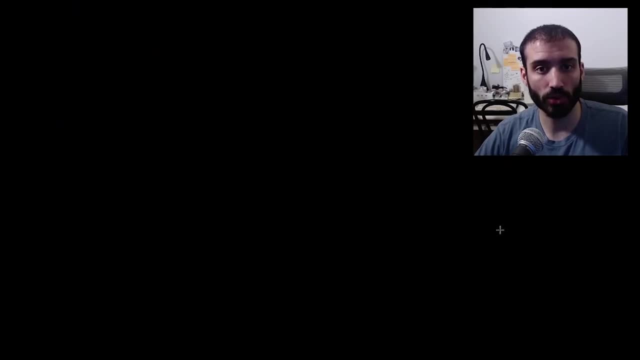 of how the singleton pattern works. Let me just make a little bit more room for myself. That looks good, All right. So there are three main benefits of using the singleton pattern First of all. all right, So there are three main kind of components of the singleton pattern, or three. 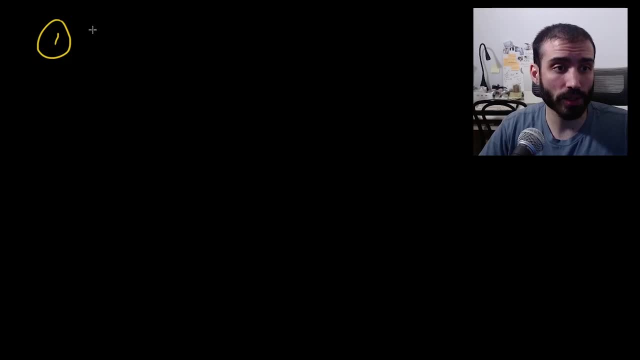 main things that you need to do to create a singleton pattern. So the first is: you have a class, It all starts with a single class, and that class needs to have a private constructor. private constructor- Well, what does that mean? Well, we're basically closing the ability of 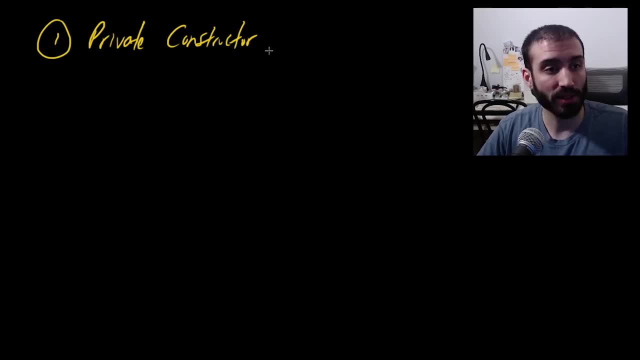 external classes to create an instance of this class. Second, we also need a private static instance of the class in question. So if our class is called food class, we need to maintain a reference to a private static instance of that class within that class. A little bit. 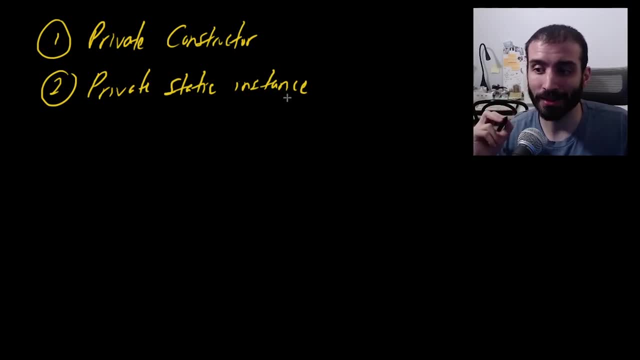 strange to talk about, but it'll make sense when you see it, I promise, And you're. you're probably wondering at this point, like if our constructor is private, how do we create an instance, or how do people even get access to an instance? That is a good question And the answer is: we have kind. 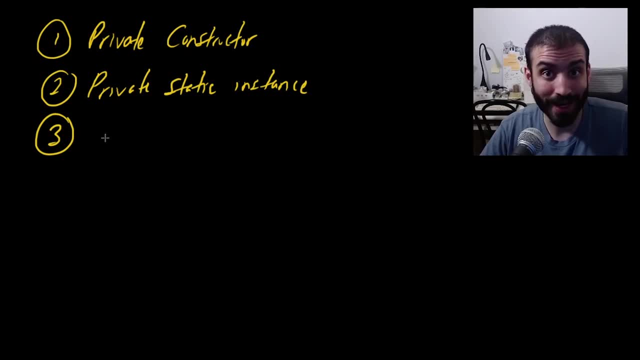 of a factory method that's responsible for creating an instance. So we have a factory method, a method for creation And, by the way, the factory method is a static method, So it's going to be at the class level: static method for creation. 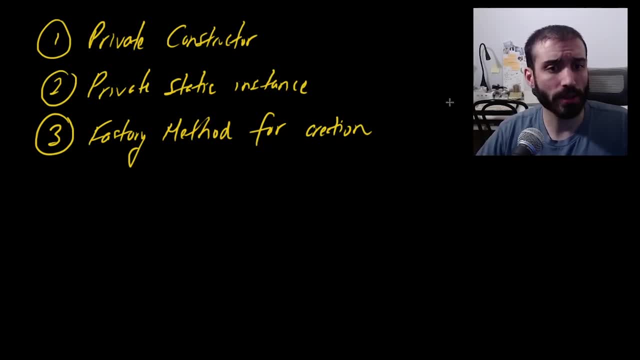 So that is all it really takes to create a singleton. You basically just have a private constructor, You have a private static instance of the class that you want to create and then you code up a factory method. and the mechanics of the factory method, like the actual code block, is super, super simple and let 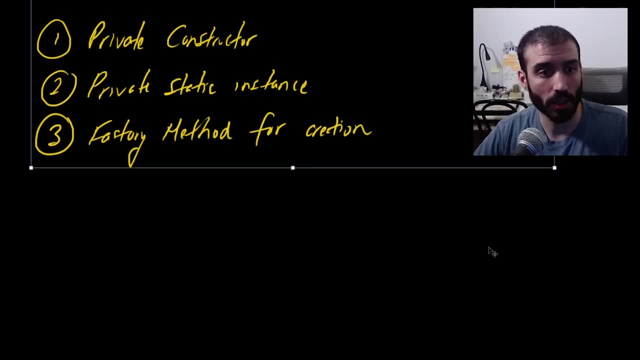 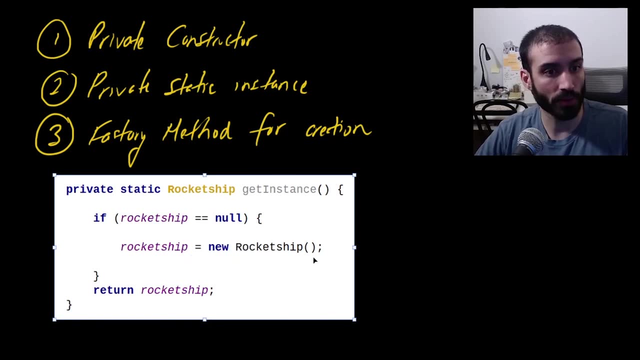 me actually just grab a picture of it here really quick so you can see what we're dealing with. so this is an example of the factory pattern of this singleton called rocket ship in this case, and it's very, very simple like: look at this: so if rocket ship is equal to null, keep in mind rocket ship. 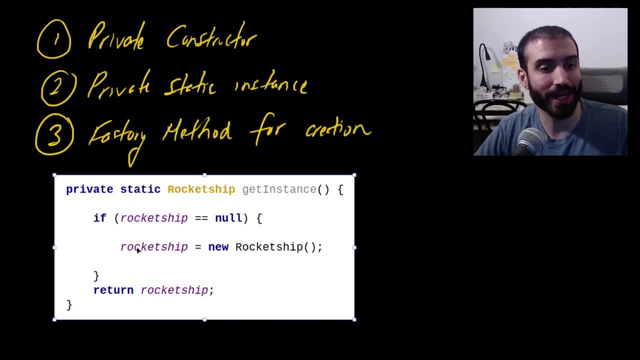 is a class level static variable. we basically just define a new rocket ship instance and then return that back. simple as can be right? not really. there's a little bit of problems with this, and the problem is it typically surfaces in the multi-threading world where you have multiple 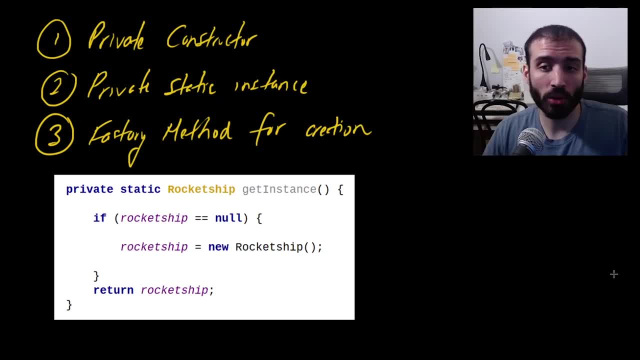 threads that are operating all at once, and so let me walk you through kind of a thought exercise of where this can become a problem in terms of multi-threading environment. so let's say we have two threads, thread one, thread one and thread two right, and these two threads are: 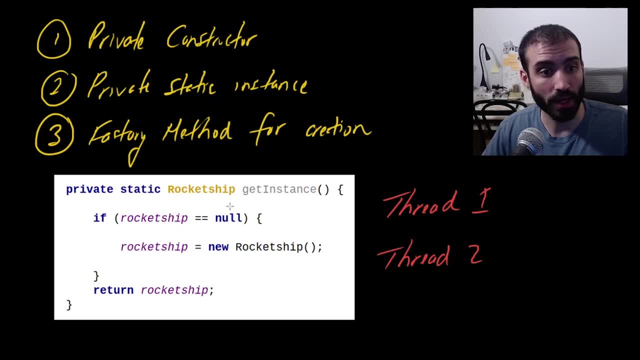 operating on the same machine and they're going to kind of want to get an instance of this rocket ship class. now, remember, in this rocket ship class it's going to be controlling a guiding system. so it is extremely, extremely important to ever only create one instance of the rocket ship and never. 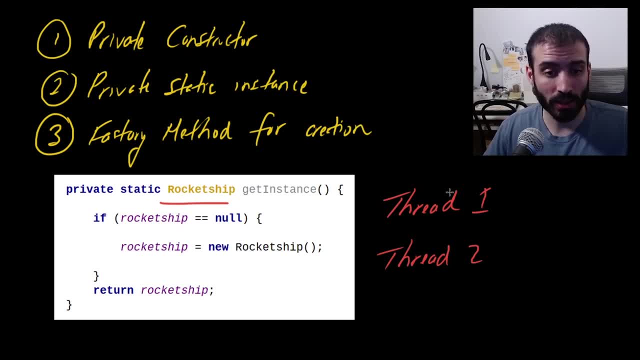 more than one. so let's consider one case here. let's consider the case where we have two threads that are trying to get an instance, so they call the get instance method of the rocket ship class. now let's say the first thread enters this code block here. so we say: you know, if rocket ship is equal to null, then we we say a rocket ship is new rocket. 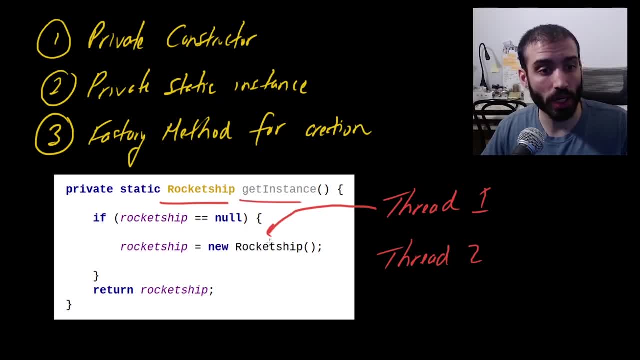 ship right. so this is the first time this get instance method is being run, so we're going to about to create a new rocket ship instance. at least that's what thread number one wants to do in this case. now what happens if we have thread number two that also enters this code: block or? 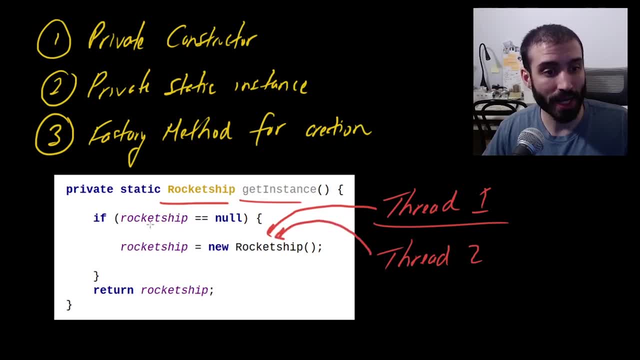 calls this method at exactly the same time. so now we have two threads that are trying to get an instance of the rocket ship class. now we have two threads right here. they've already run: if, if, rocket ship is equal to null. so they both think that rocket ship is equal to null. well then, they're going to. 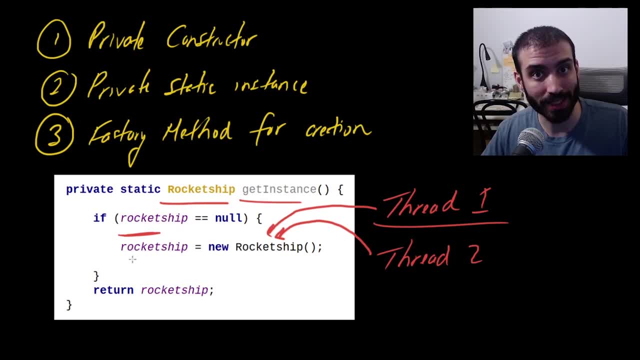 assign a new instance of the rocket ship to the rocket ship static class instance and then they're going to overwrite it and basically, whoever finished this code block last thread one or thread two- i guess it would be thread two in this case- is going to overwrite the rocket ship with. 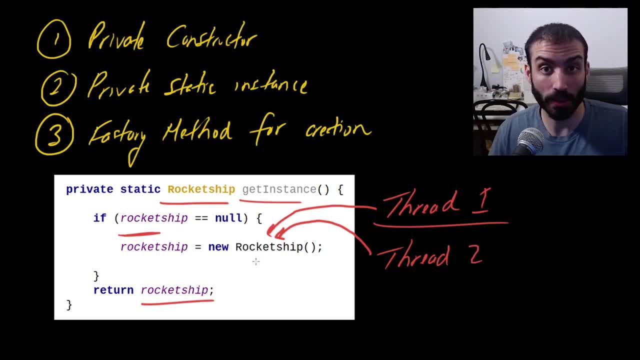 whatever instance that it created during its invocation. we saw that this is a really big problem and it's something that we can't tolerate in the singleton pattern. so this is something that you need to be careful of and how people typically solve this problem in the java programming language. 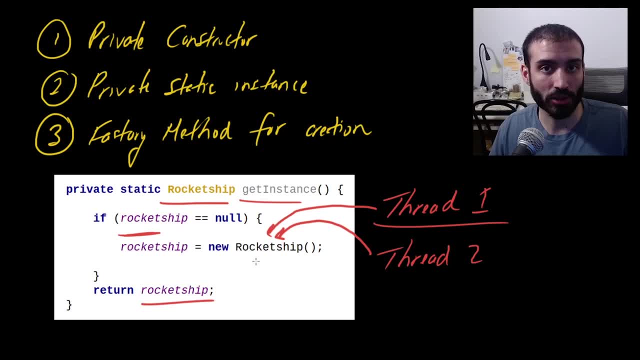 is they use what's called a synchronized block, and a synchronized block ensures that only one thread can enter a certain section of code at once, so you never actually run into this problem. so what you'd have to actually do is just kind of like put a synchronized block at this section. here you can. 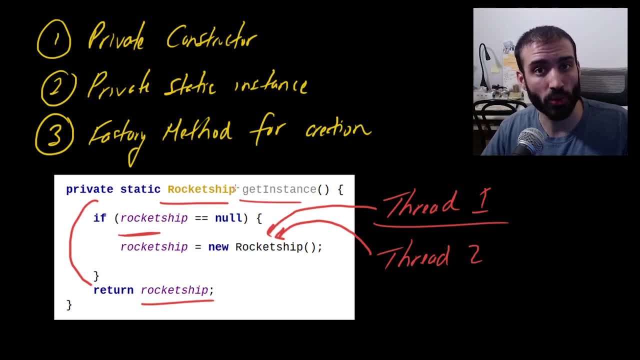 even put it on the, the class method, if you really want, but try to limit your usage of synchronize because it's a little bit of an expensive call. so really, all you have to do is add a synchronized block on this section and then you're good to go. so now we're going to run the project over and 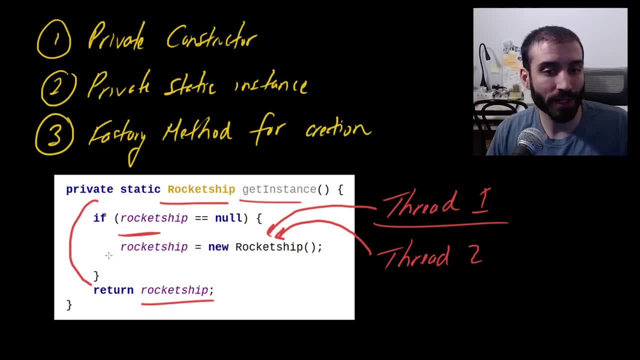 and then we're going to run the project over and and then we're going to run the project over and stuff here and then basically you're good to go. so essentially it does require a little bit of careful handling that you need to be aware of if you're going to be using the singleton pattern. 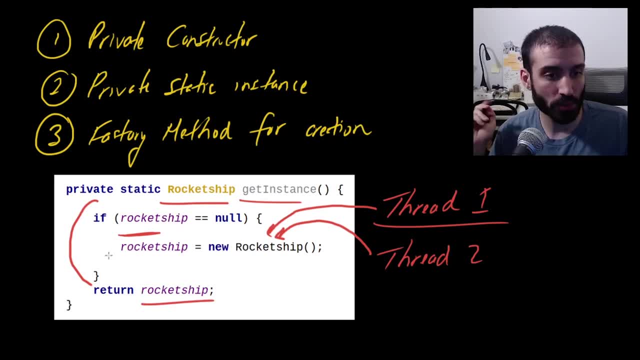 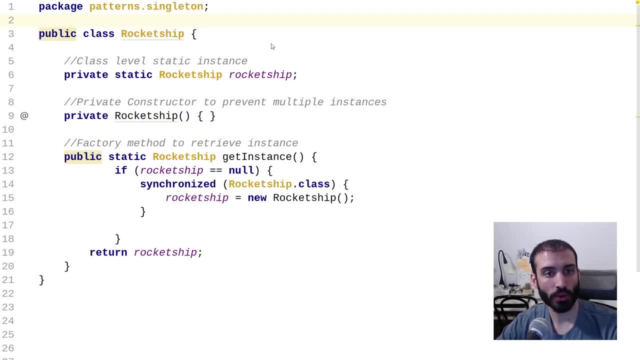 but just keep that in mind. so hopefully this part made sense. let's move into the ide now. we're going to show you an actual example of this happening. all right, guys? so here we are in the ide. so let me just walk you through some of the code that i have here, just to make this perfectly clear. 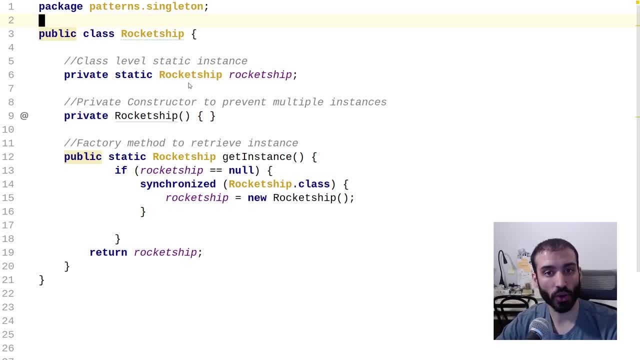 so you can see here that we have a private static instance of our rocket ship class and we're just calling that variable named rocket ship and then we're making a private constructor here of the rocket ship type that does absolutely nothing and this is the and this is intended to prevent. 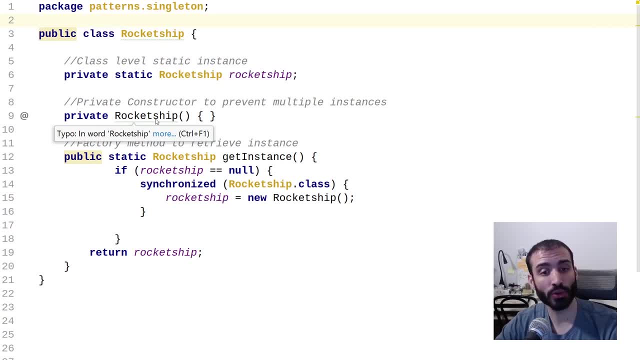 external callers from creating an instance unless they're using our factory method, which is what we have below. so here we have a public static rocket ship get instance method and the first thing we're doing is we're checking if the rocket ship instance is null. so if this is the first time entering this, 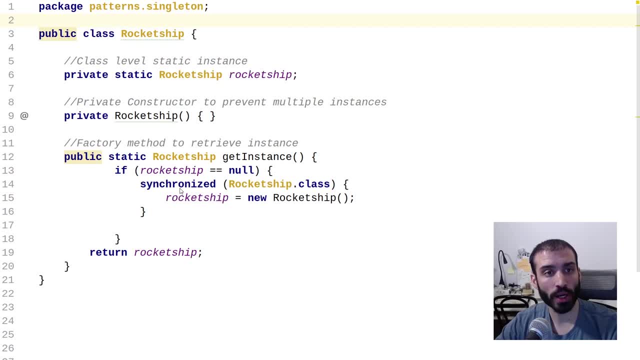 block and, as i mentioned before, we need to worry about multi-threading in the case of this rocket ship class. so we're adding a synchronized block here so that if multiple different threads call get instance at the exact same time, there's only ever going to be one single instance that ever gets created of the rocket ship. 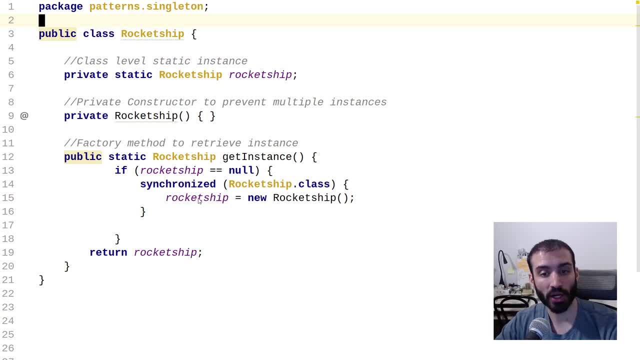 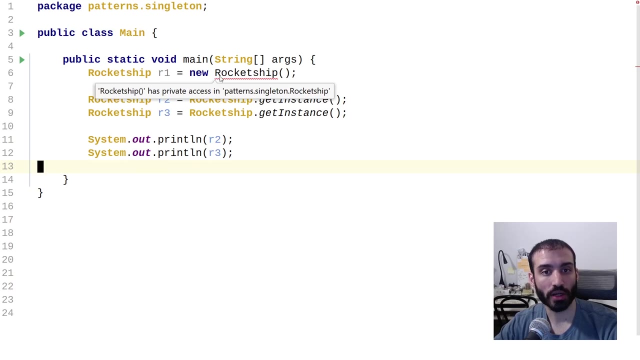 class and then we just assign the rocket ship variable to that new instance and return that back. so that is basically it for the singleton pattern. that's all you really need to know about it. so let's just take a quick little look at how this works so you can see. here i'm just trying to call the constructor and obviously my 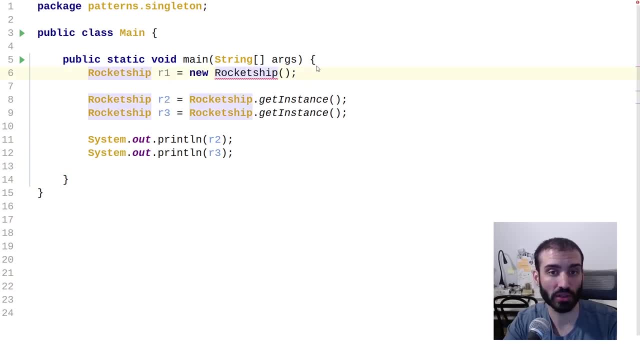 id is freaking out and complaining at me because the constructor is private, so this isn't going to work. and then what we see here is i have rocket ship r2 is equal to get instance and r3 is also get instance, and i just want to print out the lines here, just to make sure the memory addresses. 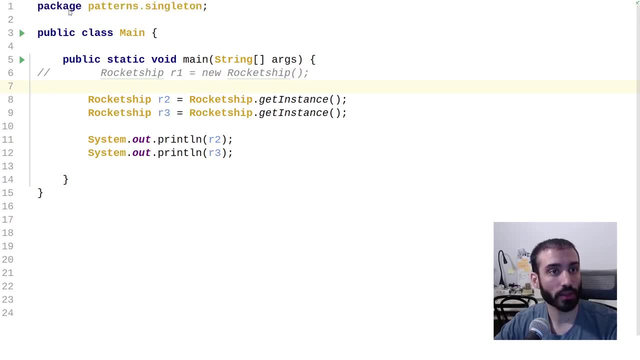 are the same to ensure that only one instance was ever created. so if we go up to run and run this guy, what we see here over on the right when we system out print line r2 and r3 is that we are printing out the same instance of the rocket ship object. so we know.